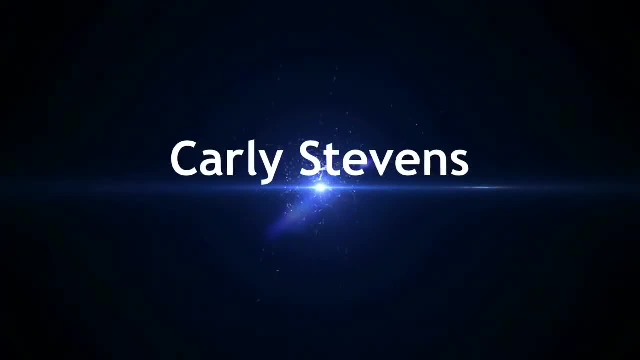 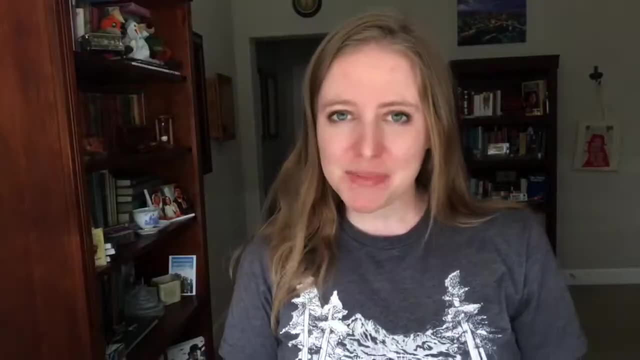 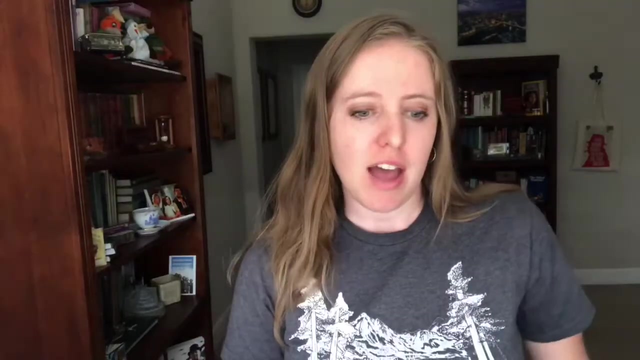 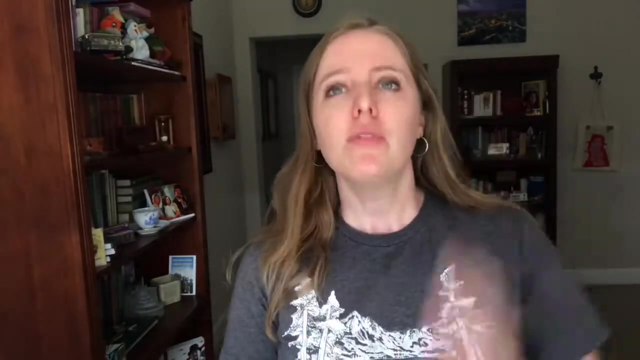 Hey, welcome back to my channel. My name is Carly Stevens and this is English Nerd, So today I wanted to give you some hacks, basically about literary analysis. Now, those words, literary analysis, can freak some people out, so it doesn't need to be frightening at all. There are some. 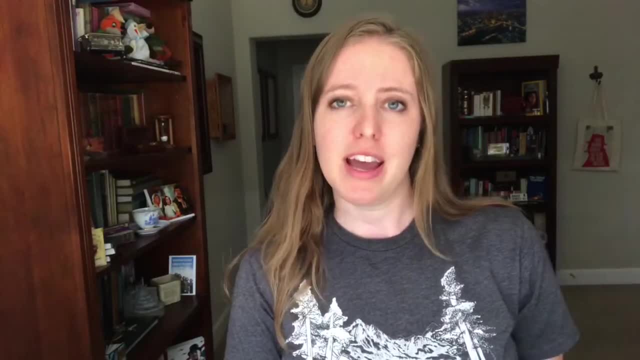 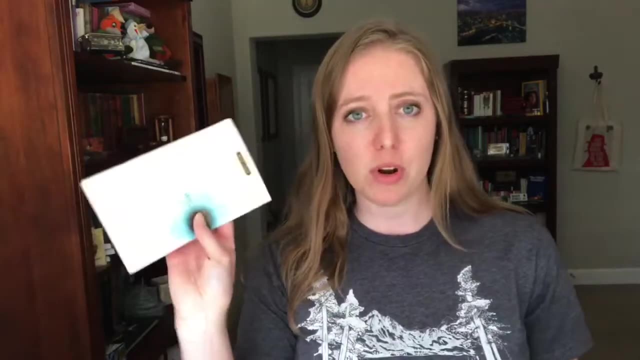 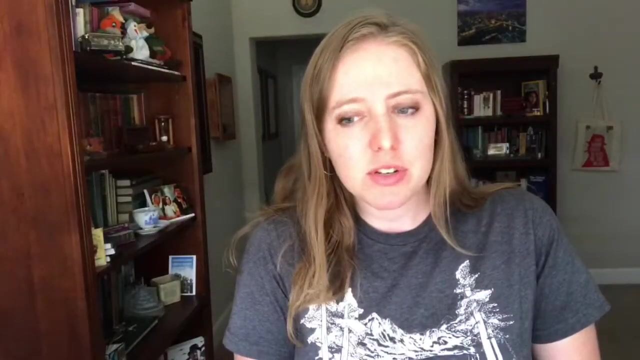 really simple things that you can do to be effective at literary analysis and getting to whatever's beneath the surface of the story. So for the example, today that's a little bright and hard to see. there we go. I'm going to use 1984. It's a really common book to 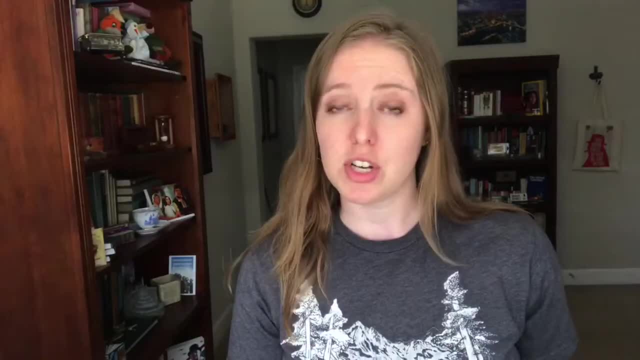 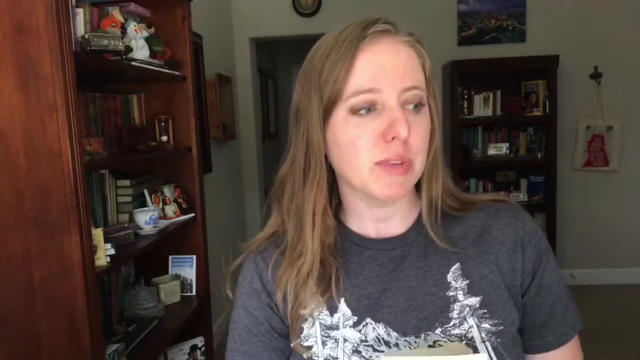 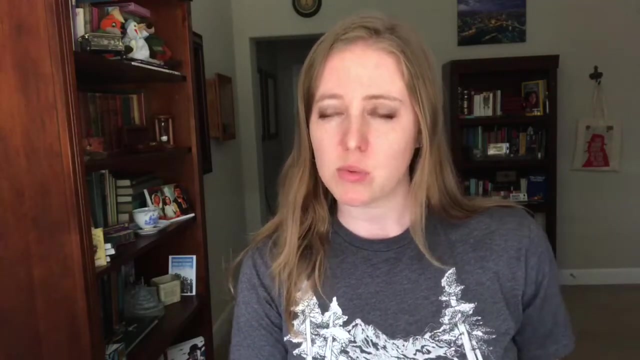 study in high school and college, and it's just really good in general. If you have not read 1984, you should by all means check it out. So the main thing I'm going to be talking about today is analyzing the beginning. If you want to get at the heart of a book, that's 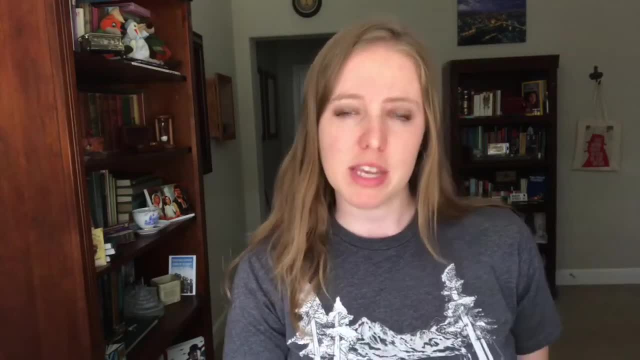 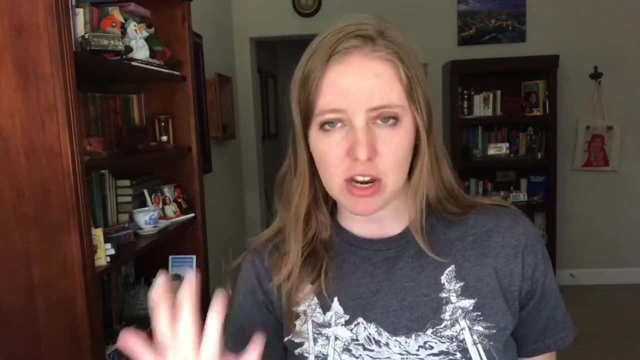 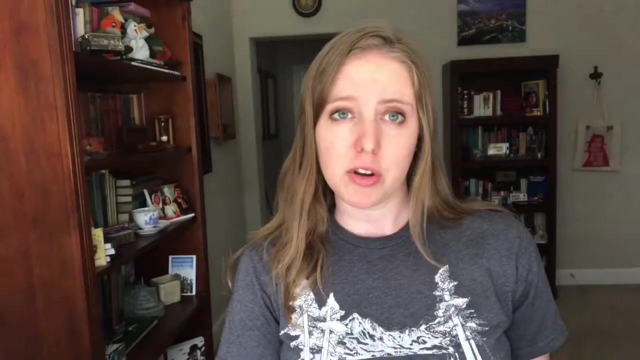 well written. you want to look closely, very closely, at the beginning and the end. Very often the beginning will encapsulate some of the themes or the tone, or sometimes the character's personalities. There is so much packed into that beginning besides just having an interesting hook. Once again, I'm sorry about the lights, They seem to be the weather's. 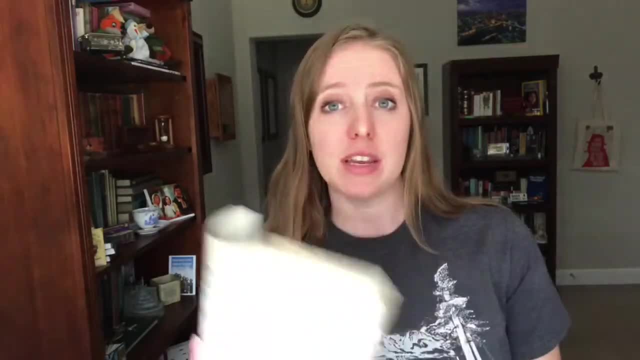 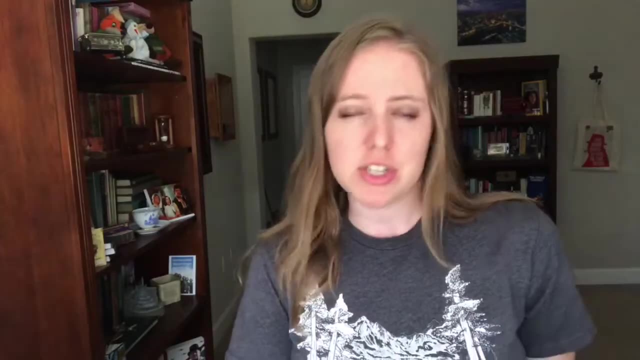 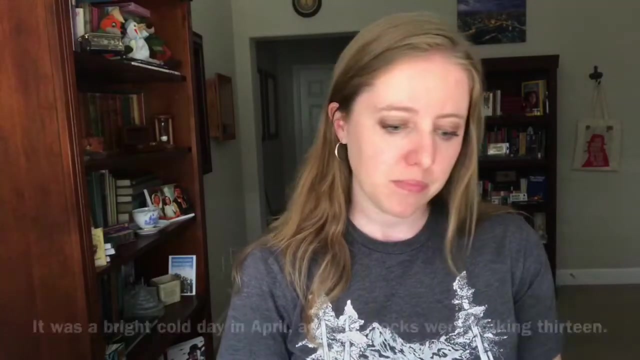 something funky. Anyway, let's take a look at the beginning of 1984 and I'll show you how you can do some literary analysis even on your own, if you're not an English teacher or some kind of expert. 1984 by George Orwell begins this way, very famously: It was a bright, cold day in April. 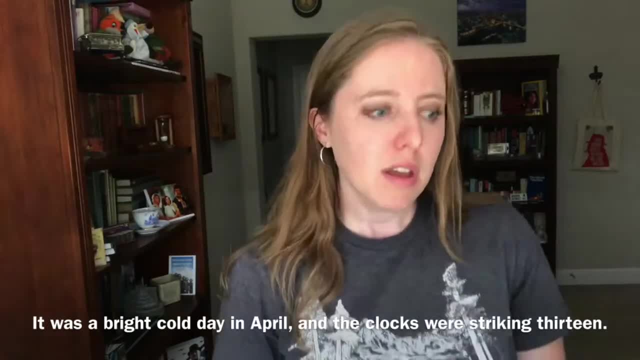 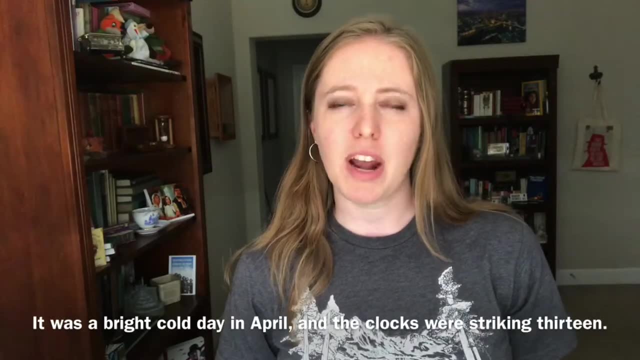 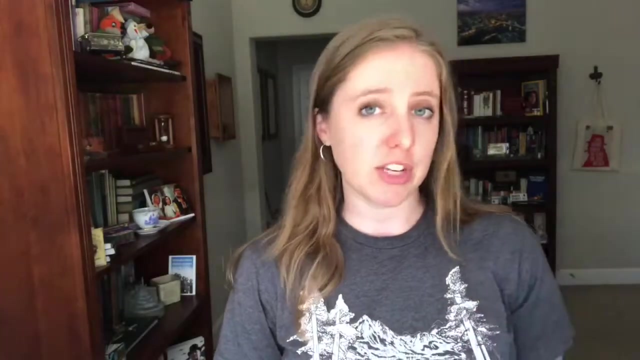 and the clocks were striking 13.. Now you don't need to be any sort of English wiz to realize that there is a There's something off about having the clocks strike 13.. The key to good literary analysis is just observation. That's it. It's just observation. So let's think about that idea. 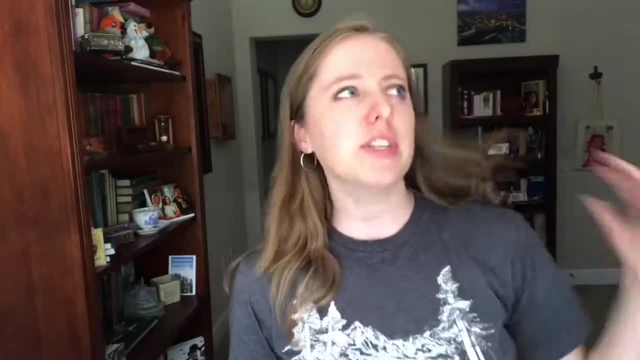 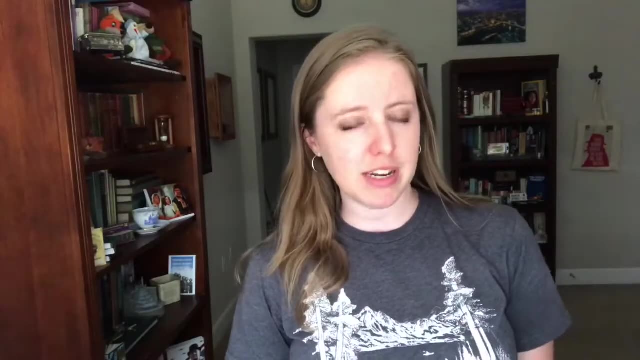 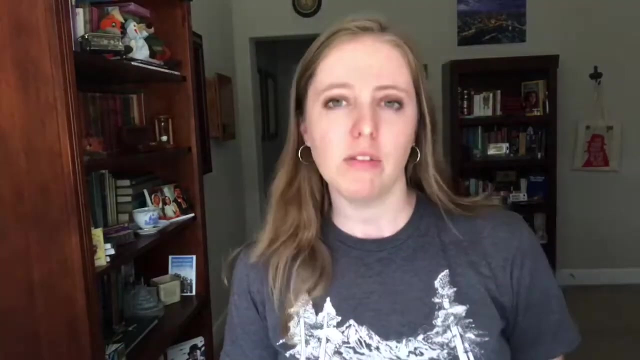 that the clocks were striking 13.. Okay, so 13 is considered by many cultures to be an unlucky number, which is why we have no floor 13 in most hotels. So 13, we have an unlucky number. We have one number above 12,, of course, which means that we are probably on military time. 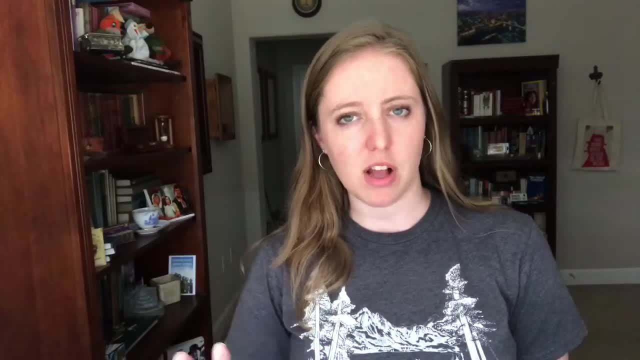 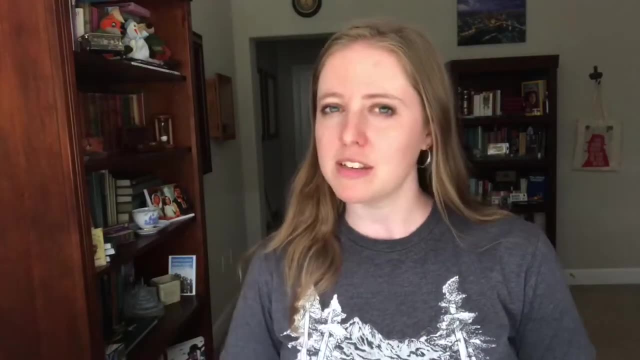 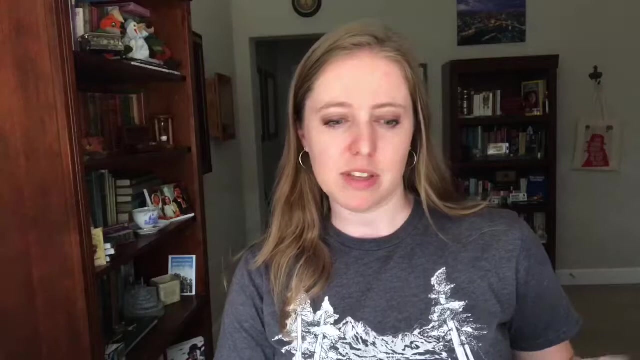 So already we have this slightly unsettling feeling that the clocks are striking 13,, that unlucky number, and that means that we're probably on military time for some reason. And the question becomes: what is that reason? Is this a militaristic society or what So? 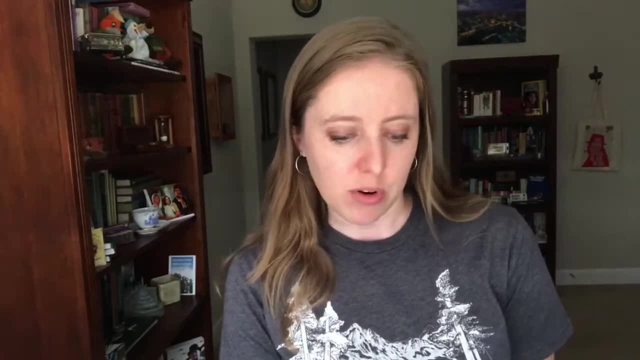 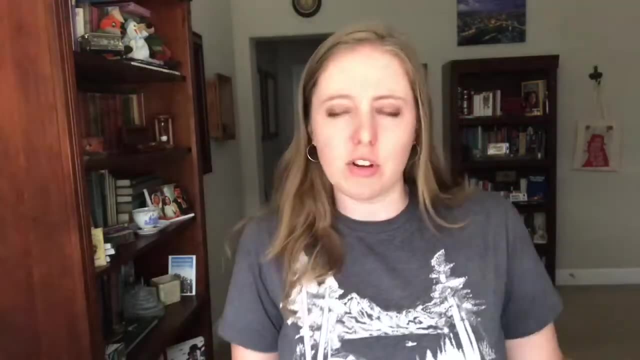 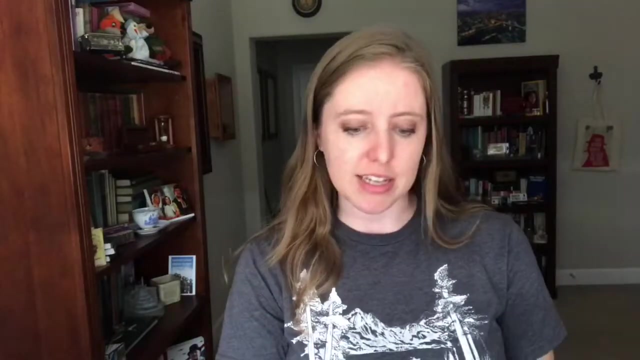 it's a bright, cold day. It's a cold day in April. Everything seems fine, but then there's that turn, that twist, And we got all of that just from thinking. the clocks are striking 13.. Hmm, interesting. So you have something to work with now If you go on to the second sentence, which brings 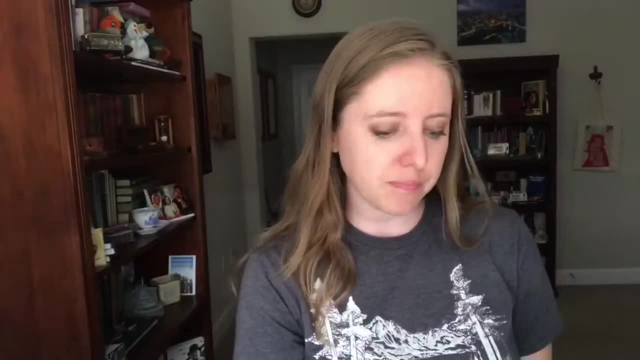 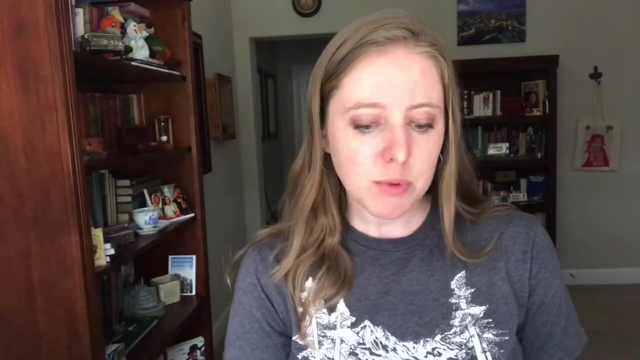 you to the end of the first baby paragraph. there it says this: Winston Smith. his chin nuzzled into his breast in an effort to escape the vile wind, slipped quickly through the glass door, And then he climbed over the last doors of Victory mansions, though not quickly enough. 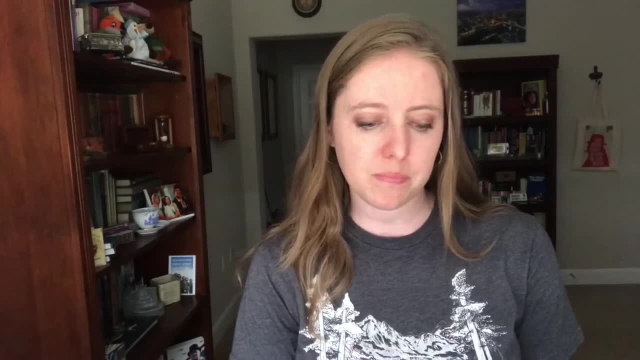 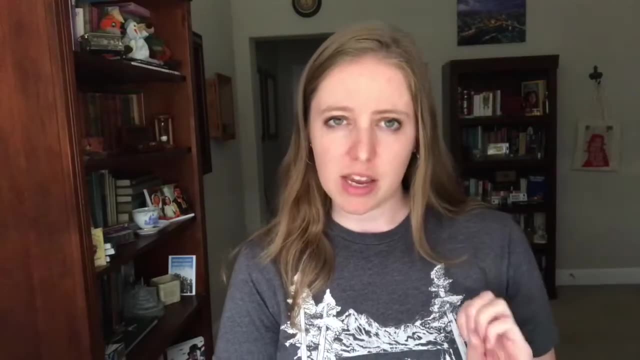 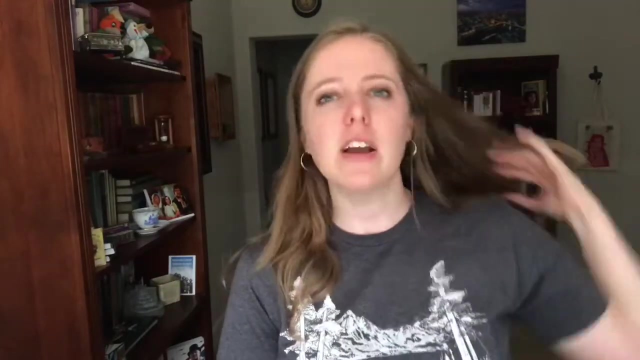 to prevent a swirl of gritty dust from entering along with him. OK, So you, as the literary analyst, will start picking out some of those details, like the name of the protagonist, Winston Smith, for instance. Smith is a really common last name. 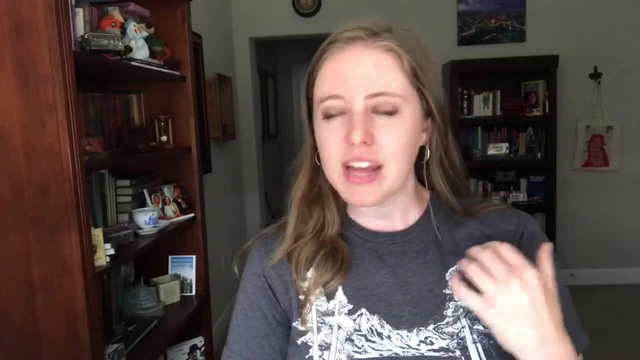 Maybe there's something to that. Maybe—anytime you have a character whose name ends with Smith or begins with Smith, maybe you'll know that they're both a little more kinds of names. Do you know more about that? Do you, Do you? 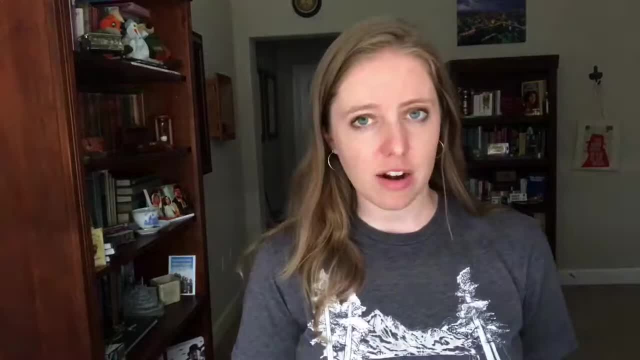 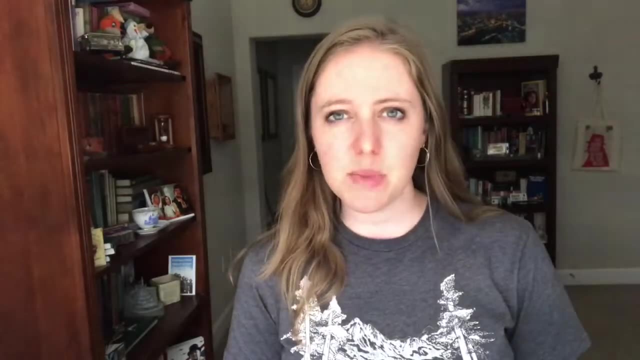 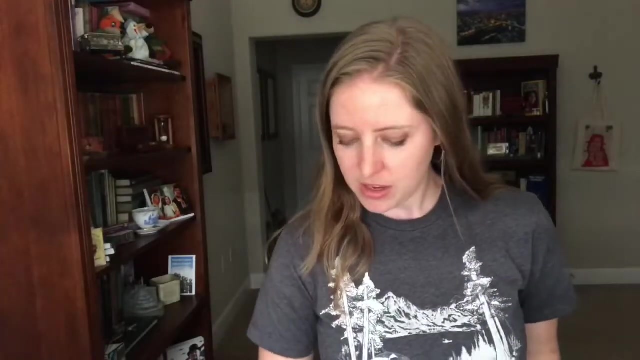 with some form of John. chances are, if it's you know great literature, that you're looking at an everyman kind of character, And Winston Smith is set up anyway to potentially be that kind of character. The name Winston is also interesting. This book was written in 1950, and so that was. 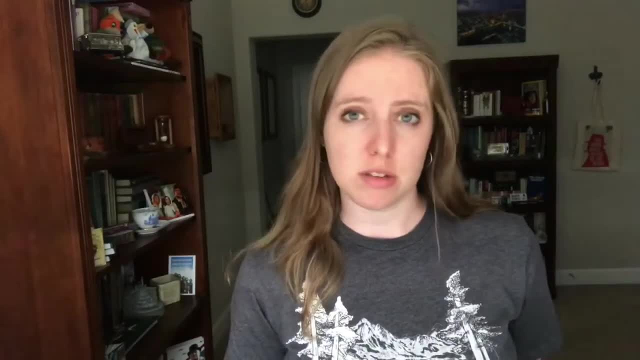 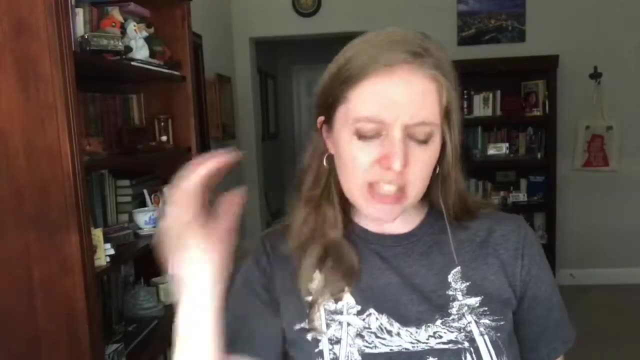 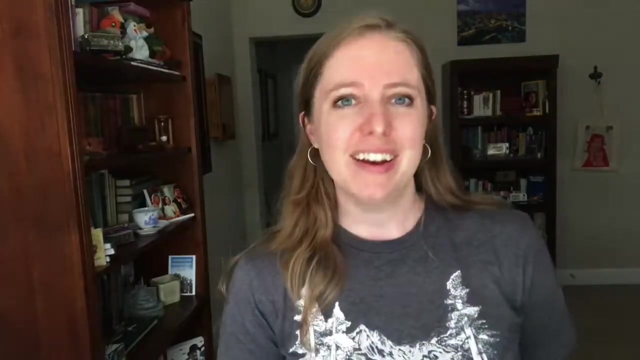 within very recent memory of World War II, Stalin was still in charge. This book, of course, is going against Stalinist ideas. Winston would bring to many people's mind Winston Churchill. If you see, right here I have a Winston Churchill bag. He's a fascinating guy. So there's this sense. 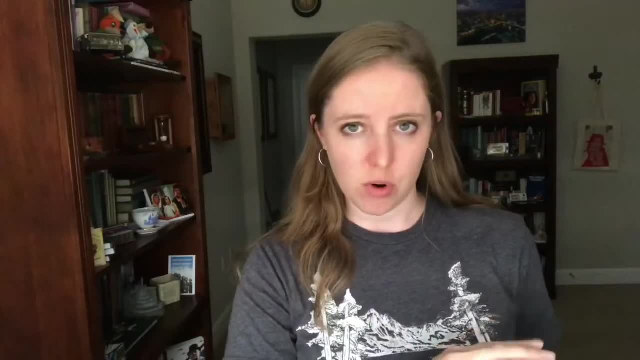 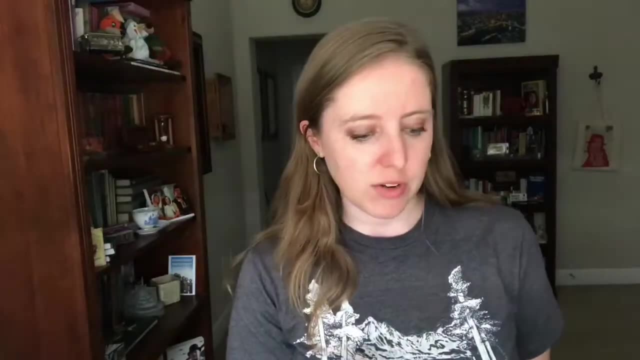 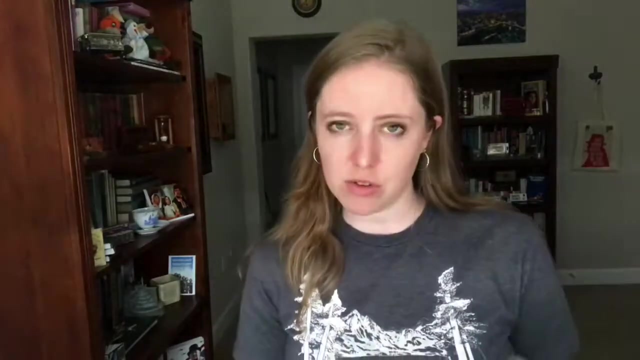 that we have an everyman, but with the potential for some kind of greatness perhaps. But it says his chin nuzzled into his breast in an effort to escape the vile wind, slipped quickly through the glass doors of Victory Mansions. Maybe Victory Mansions stood out to you the first time. 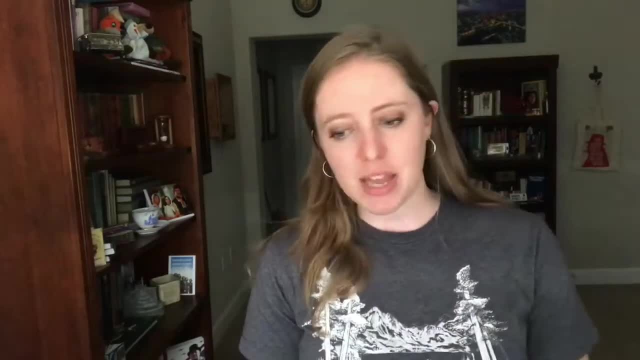 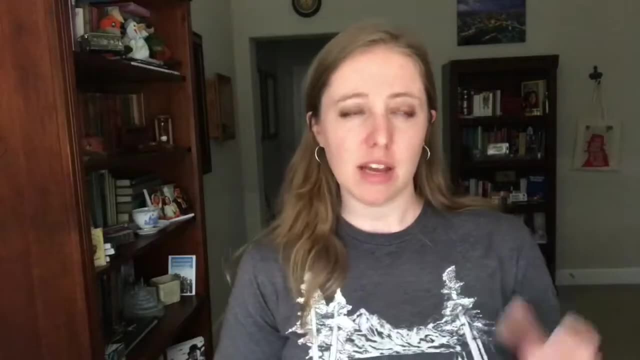 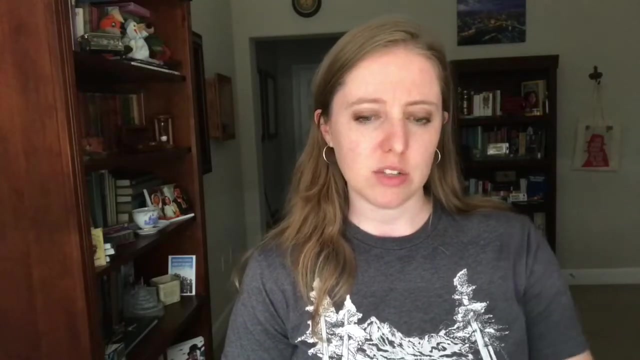 you read this or that? I read it to you. We have Victory Mansions, but vile wind taking gritty dust comes in with Winston, So something's again not quite matching up, Something's called Victory Mansions, but it sounds not so nice. All this gritty dust is swirling in behind Winston, So all of 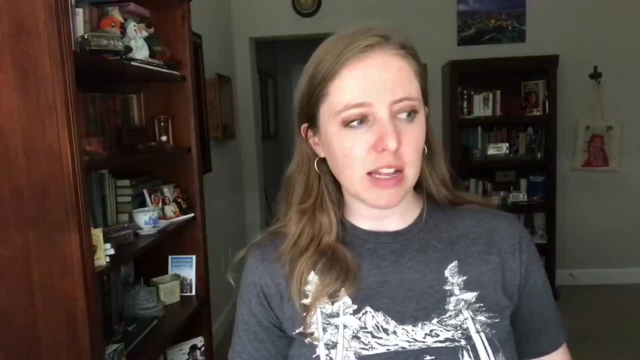 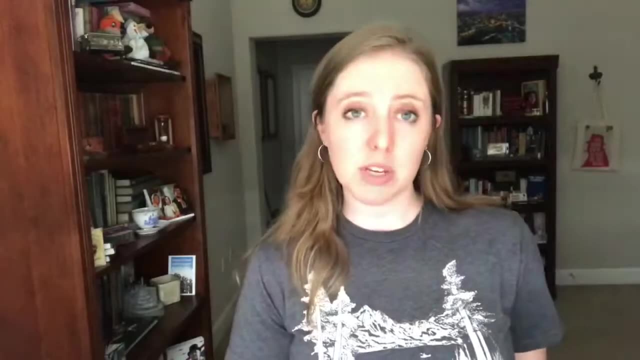 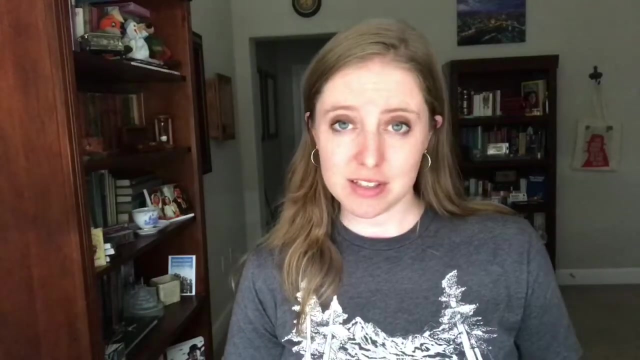 these things. these first two sentences set up this unsettling militaristic things appear to be one way, but actually are another tone, as well as something about the protagonist, Winston Smith. Just by his name alone, we, at least, can have the hypothesis that he might be an everyman character, with the potential for greatness, Of course all. 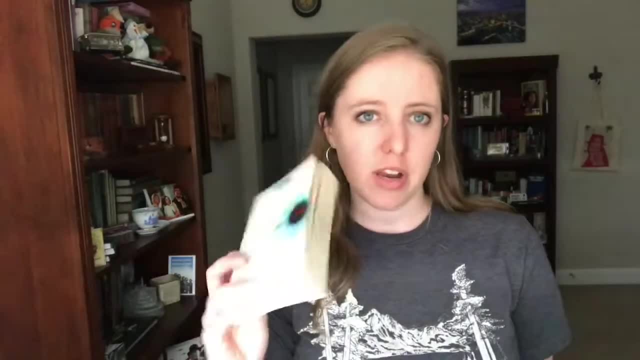 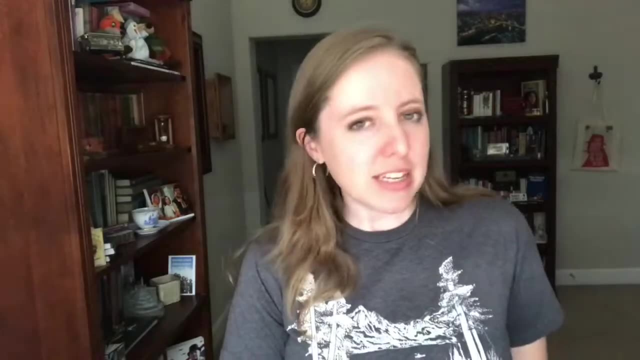 these things, we need to see how they would play out in the book as a whole. You can't just look at the beginning and go to your test and say, yeah, I'm set to go. You do need to see if those things pan out. 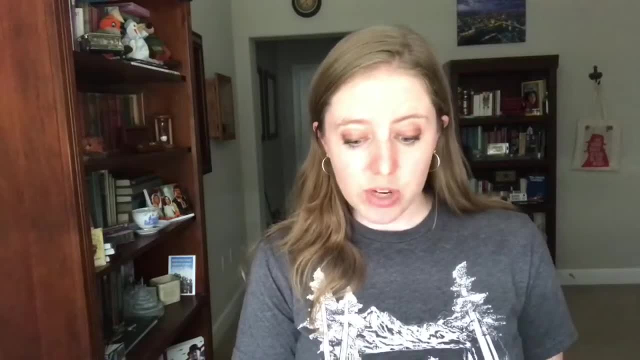 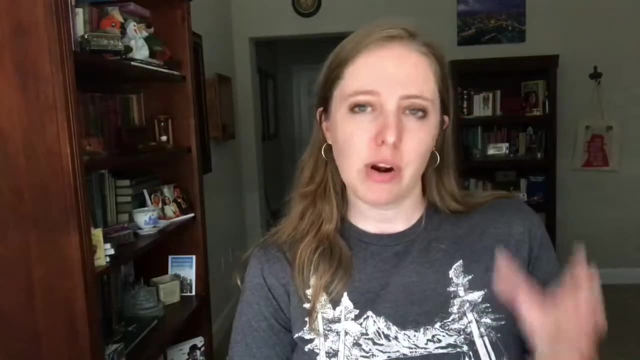 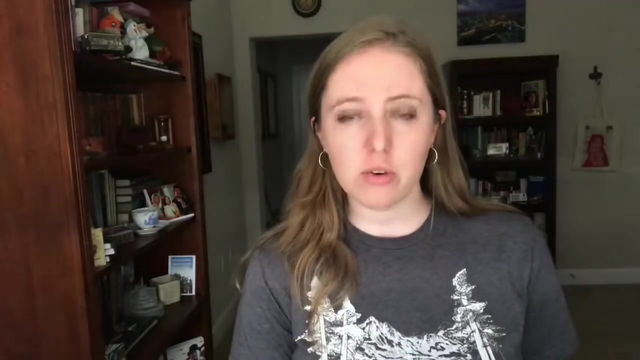 Or if they're meant to be ironic and things like that. But that is one really simple way that you can be basically a pro-level literary analyst, no matter who you are. Look at the first couple sentences of whatever work that you're reading- the poem or novel or whatever- and pick it apart. 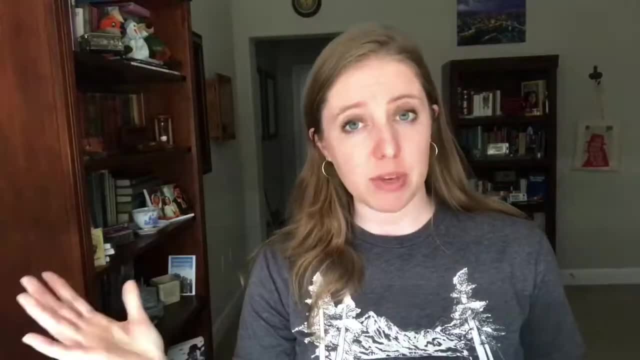 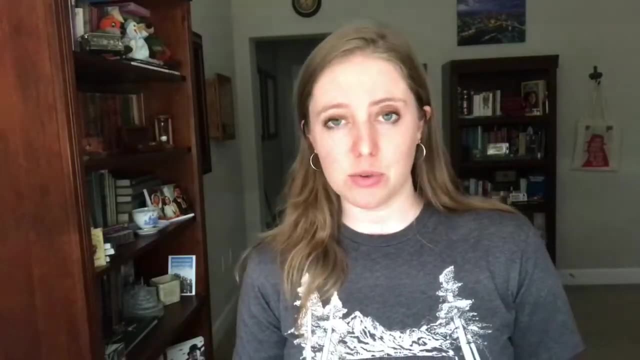 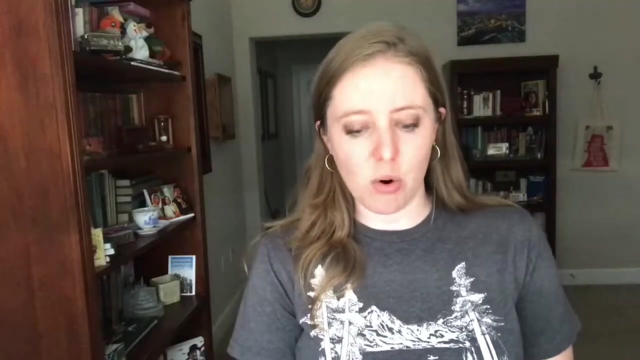 Observe and then think: well, why might that be? That's it. That's it. Literary analysis is just that, taken to an extreme. So you have everything you need to be successful at this, no matter which class you're taking Or if you just want to get better at understanding.